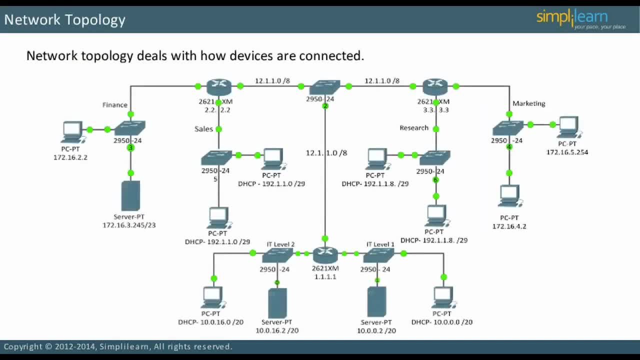 slide. As shown in the image on the slide, network topology deals with how devices are connected to each other. As shown in the image on the slide, different devices in finance, IT level 1,, IT level 2, and marketing are connected through a network. This is dependent on the technology available. 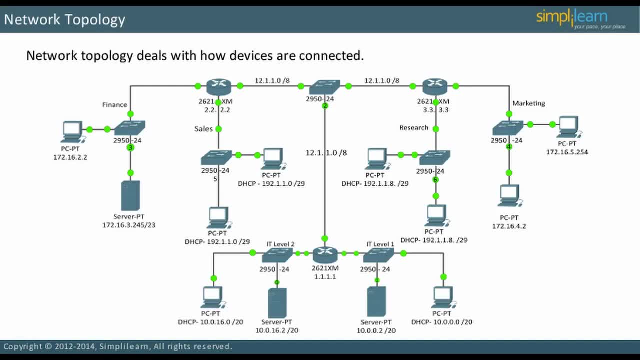 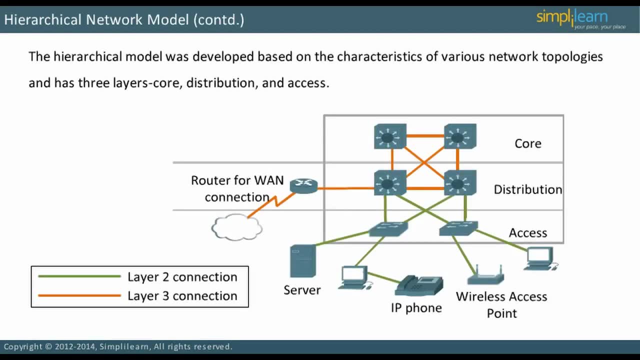 Network topology is categorized into few types. We will be looking into them one by one in the following slides. The image on the slide depicts how each layer fits together in the network. As discussed, the hierarchical model is defined by the characteristics of the network topologies. It has three layers: core distribution and 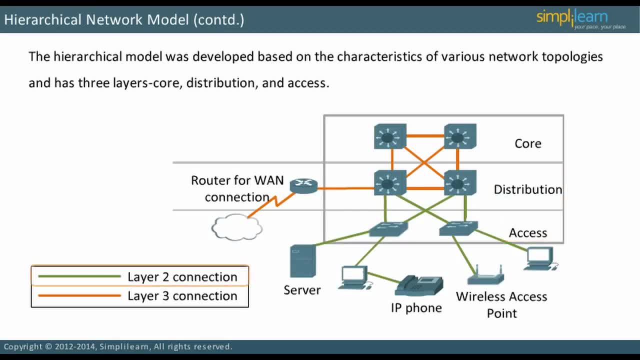 access. There are two types of connections that link the devices. They are Layer 2 and Layer 3 connections, As depicted in the image. both these connections are present between the devices. Note: the Layer 3 connections end at the distribution layer. Below that, all connections are Layer 2.. The rest of the connections 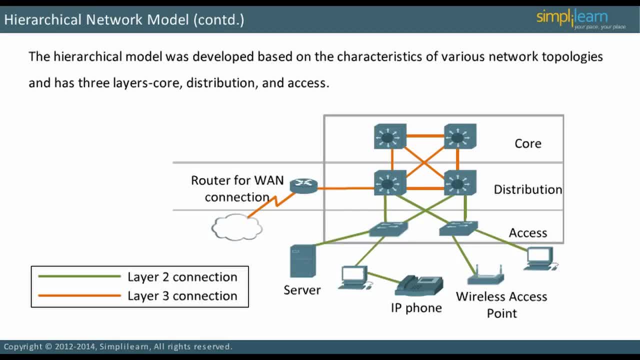 end at the distribution layer. In the image, the router connects to a remote network. This is a Layer 3 connection Distribution and core layers are linked through Layer 3 connections. The switches in both these layers are multi-layer switches or MLSs. 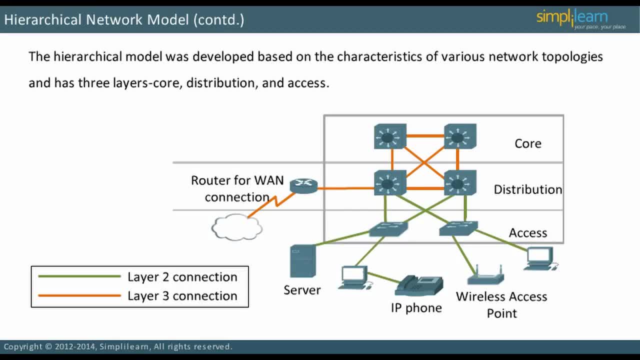 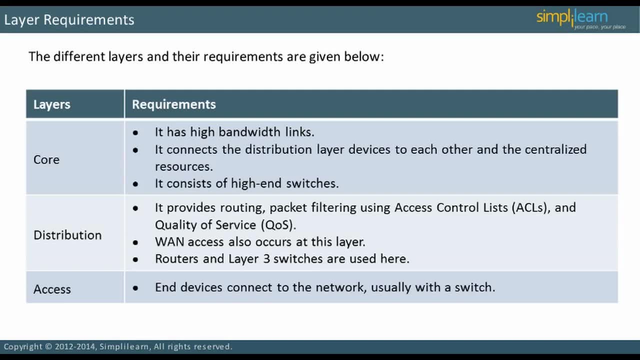 These can do: Layer 3- routing, and Layer 2- forwarding. Let us discuss the layer requirements in the following slide. The different layers and their requirements are as follows. The core layer has high bandwidth links. It connects the distribution layer devices to each other and the centralized resources, such as database. 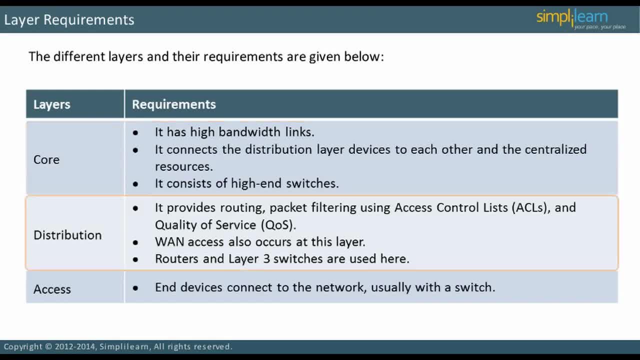 servers. The core layer consists of high-end switches. The distribution layer provides routing, packet filtering using access control lists and quality of service. Wide area network access also occurs at this layer. Routers and Layer 3 switches are used here. The access layer is where end devices connect. 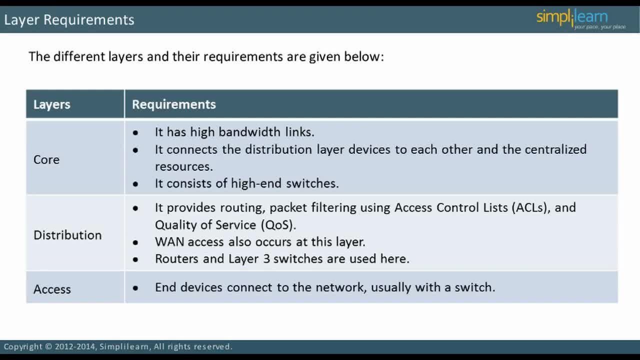 to the network. Let us focus on an important Layer 1 and 2 technology, that is, Ethernet, in the following slide.